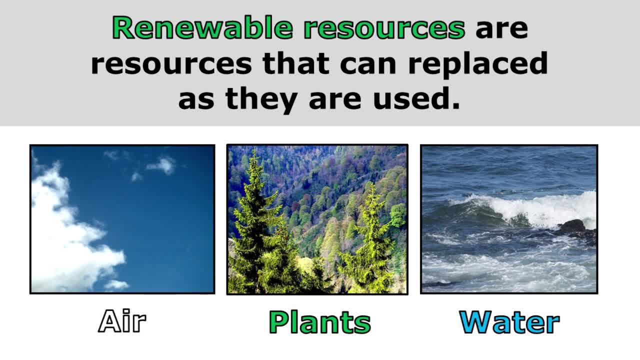 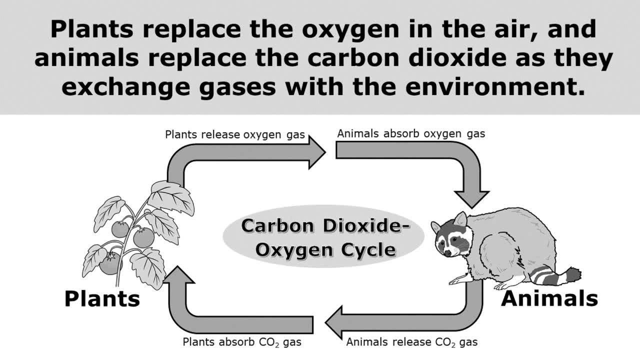 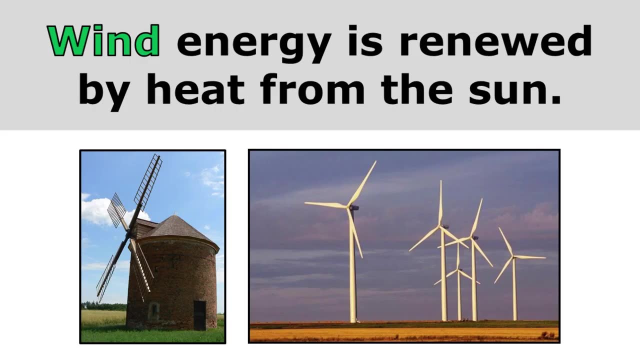 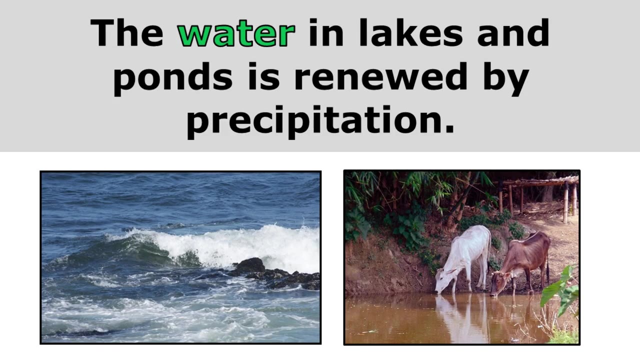 Air, plants and water are all examples of renewable resources. Plants replace the oxygen in the air and animals replace the carbon dioxide as they exchange gases with the environment And wind. energy is renewed by heat from the sun. The water in lakes and ponds is renewed by precipitation. 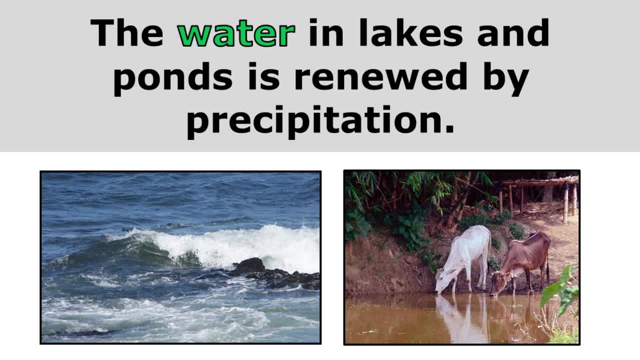 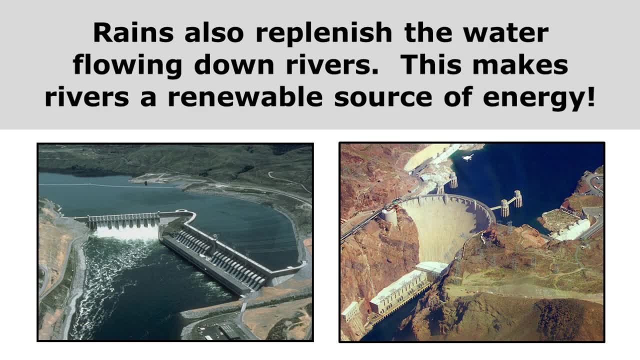 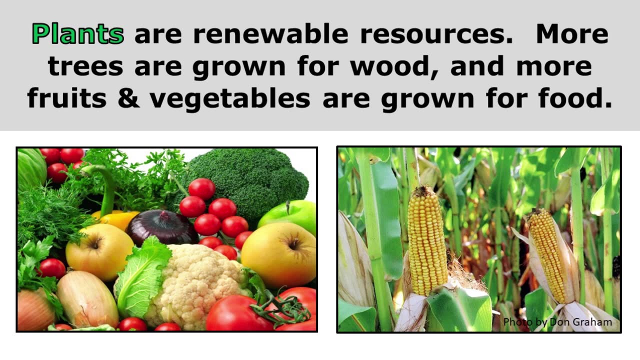 The rain replaces the water that's produced. The rain replaces the water that's been used. Rains also replenish the water flowing down rivers. This makes rivers a renewable source of energy. Plants are renewable resources. More trees are grown for wood and more fruits and vegetables are grown for food. 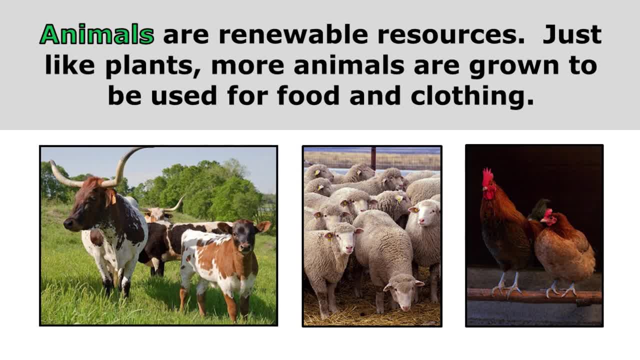 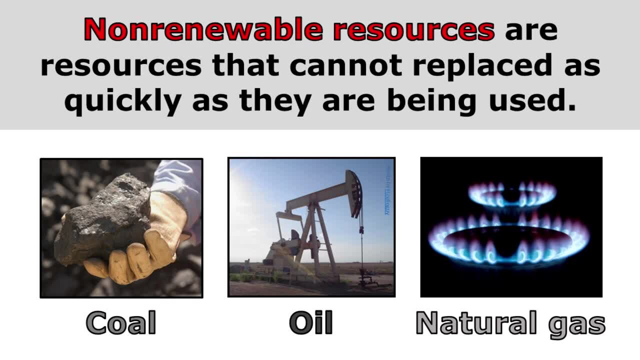 Animals are renewable resources too, Just like plants. more animals are grown to be used for food and clothing. Non-renewable resources are resources that can be replaced as they are used. Non-renewable resources are resources that cannot be replaced as quickly as they are being used. 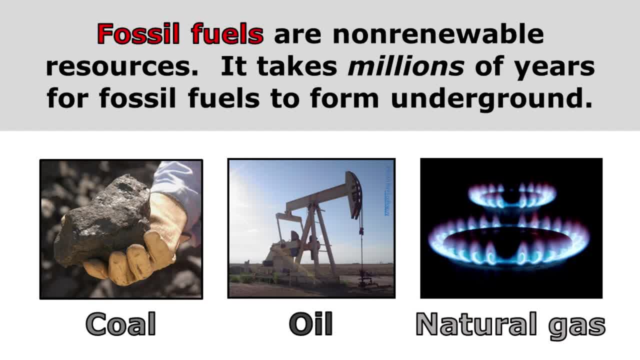 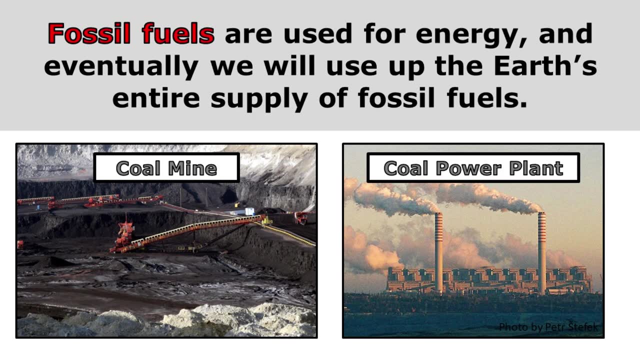 Fossil fuels are non-renewable resources. It takes millions of years for fossil fuels to form underground, So coal, oil and natural gas are all fossil fuels that are non-renewable resources. Fossil fuels are used for energy and eventually we will use up the earth's energy. 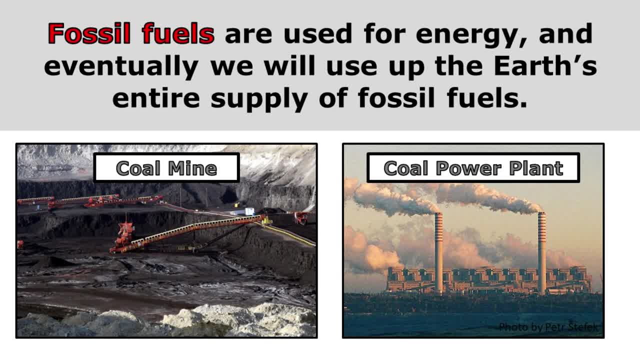 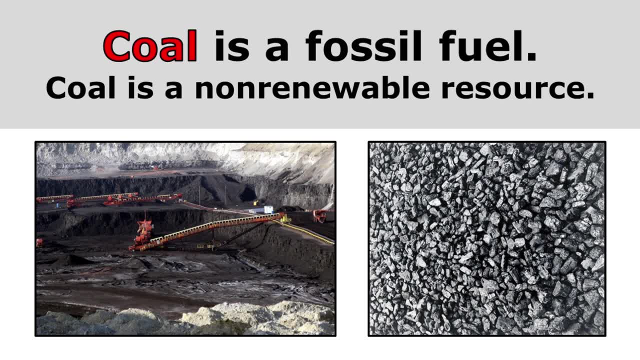 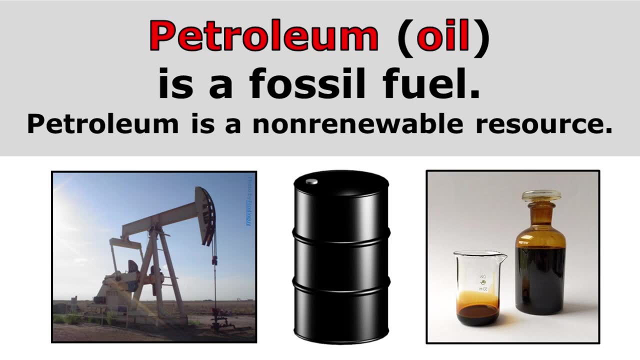 And eventually we will use up the earth's energy. And eventually we will use up the earth's energy. Coal is a fossil fuel and a non-renewable resource. Petroleum, or oil, is a fossil fuel. Like all fossil fuels, petroleum is a non-renewable resource. 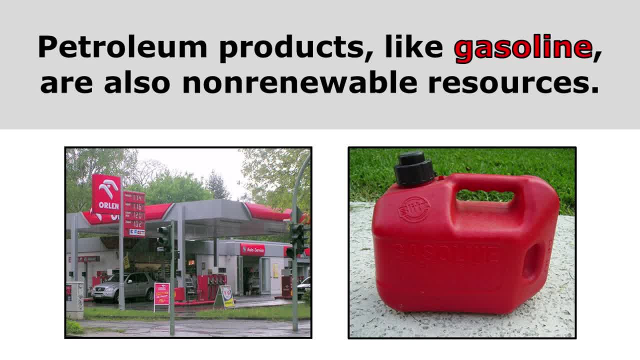 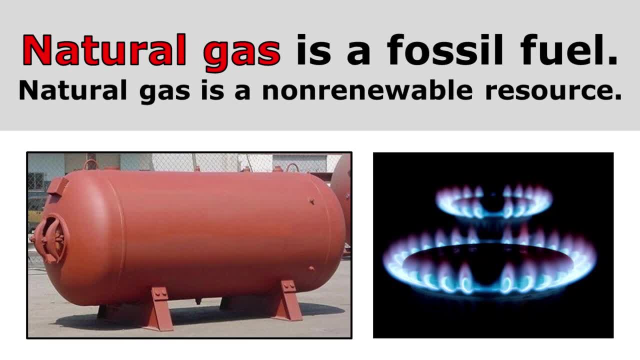 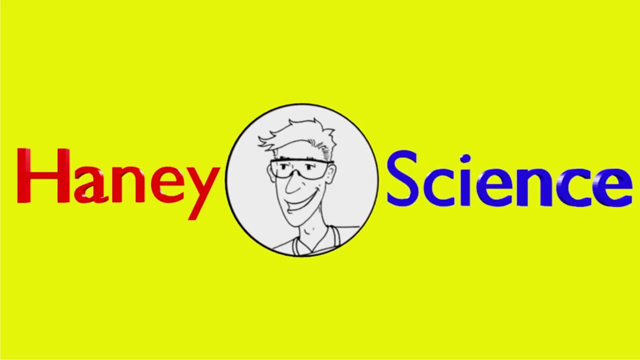 Petroleum products like gasoline are also non-renewable resources, And natural gas is a fossil fuel, So natural gas is also a non-renewable resource. So natural gas is also a non-renewable resource. So I hope this video has helped you understand renewable and non-renewable resources a little better. Keep up the great work and I'll see you next time.